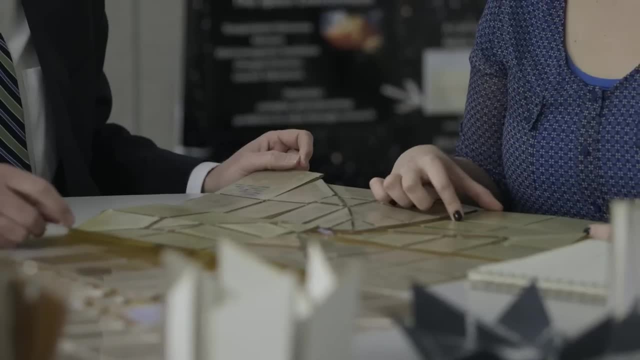 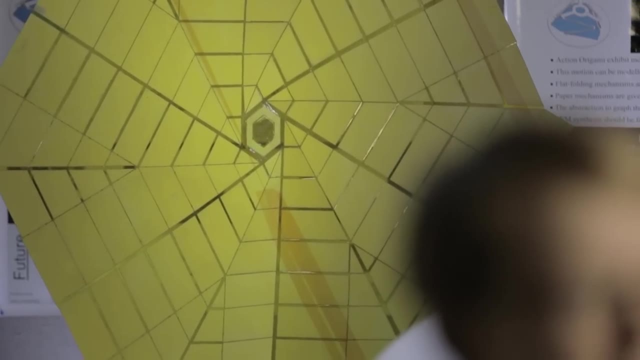 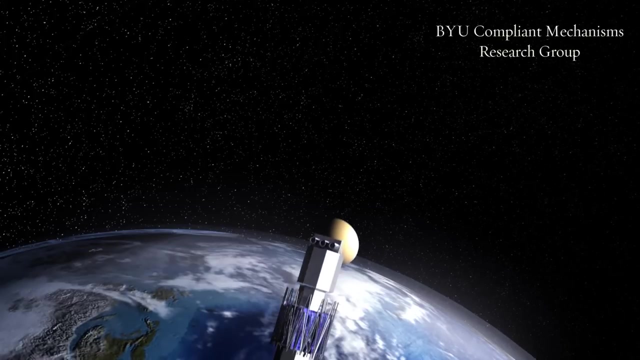 You get into space, you can deploy and be very large. I'm working on an origami-inspired deployable solar array for a spacecraft. The panel hanging behind me is the 20th scale prototype of this 25-meter array system By using origami principles. 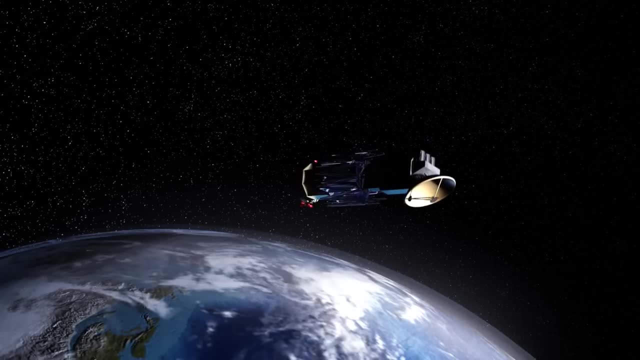 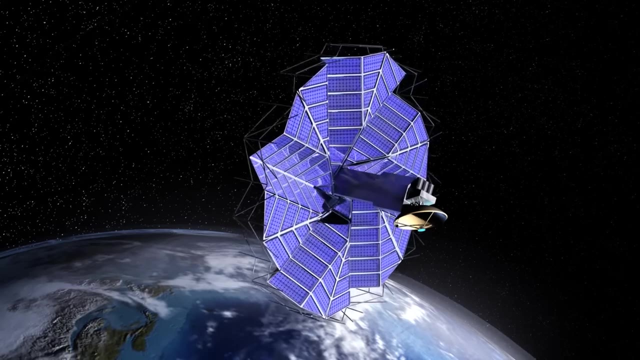 we can get a much larger array into space by stowing it compactly during launch and then opening it up once we're in space. The spacecraft would be inside a rocket, like an Atlas 5. And the solar array would wrap around the outside of the spacecraft and it would be 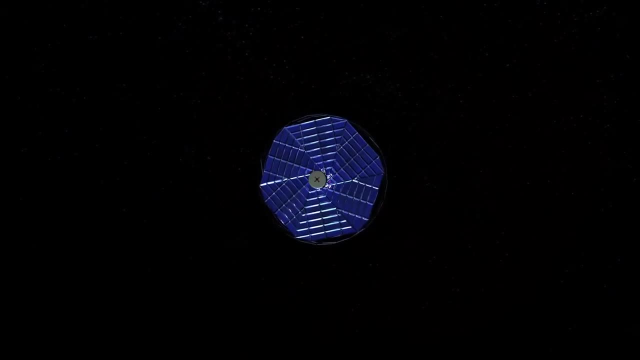 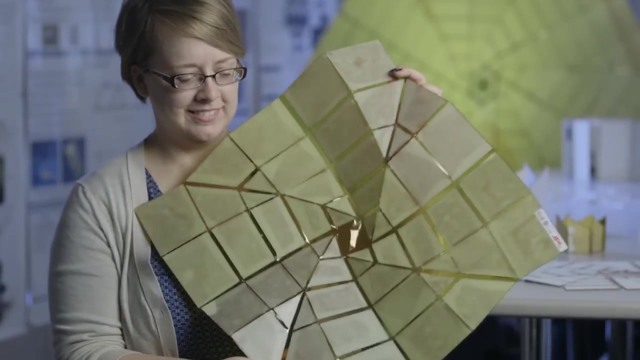 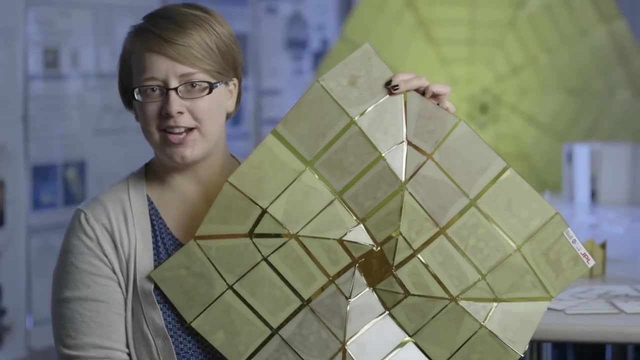 all folded up compactly and then launched into space and deployed. This is our CubeSat version. As we open it, it opens to about 50 centimeters and has the potential to generate about 65 watts of energy at this actual size. CubeSats are kind of the new, novel way of getting things into space quickly, because 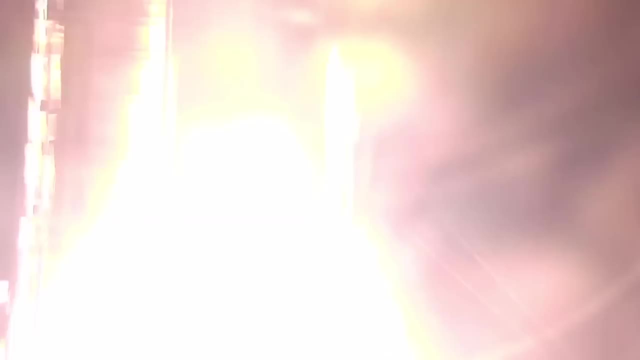 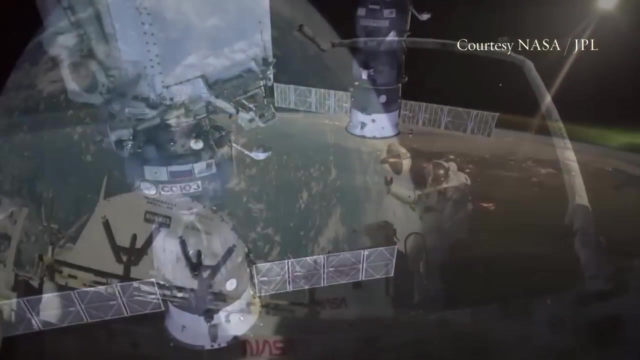 they're small, They don't cost a lot and you can throw them on with any rocket that's going into space. In addition to working with people like the National Science Foundation, we have projects with NASA Marshall Space Flight Center in Alabama and also with the JPL. These are the 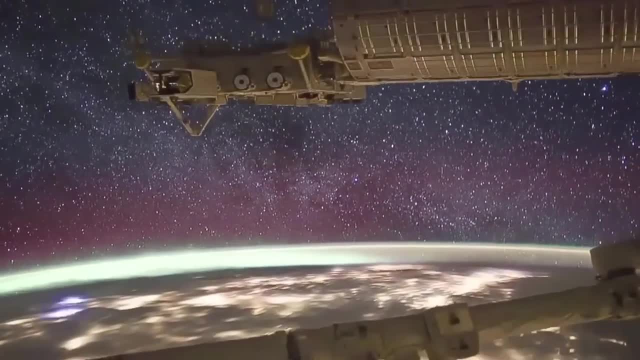 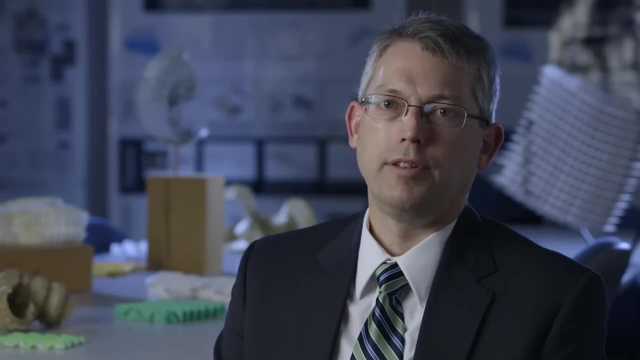 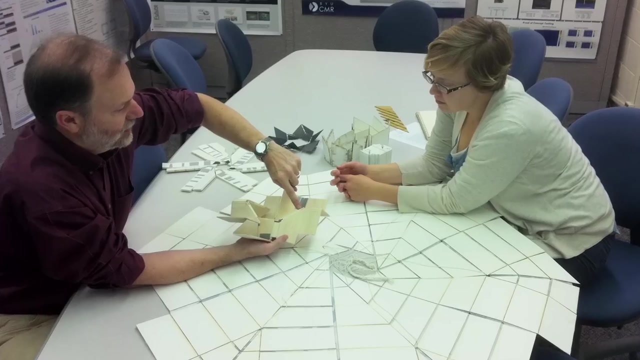 same people that do the Mars Rover and other things We are doing: origami-inspired mechanisms, expanding solar array. We're involved with a collaborator, Robert Lang, who is a world-renowned expert in origami. It's very unique to work with someone who is such an expert. He's defined an area for 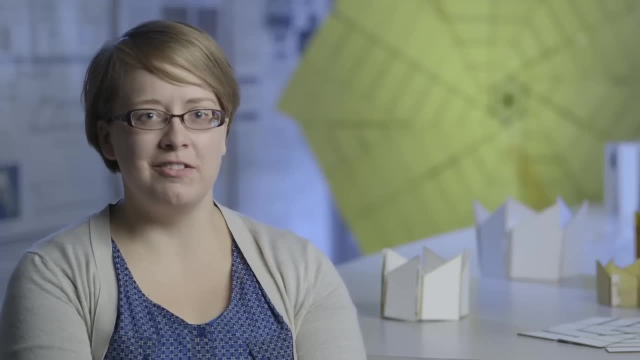 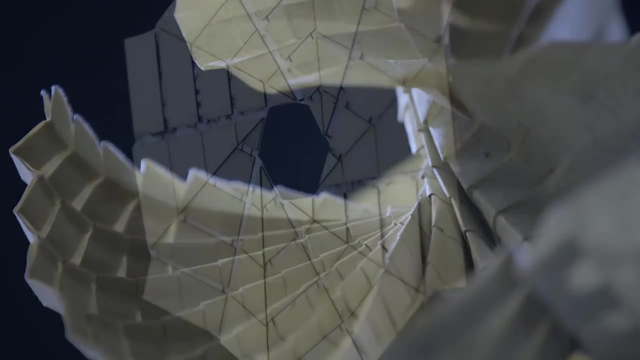 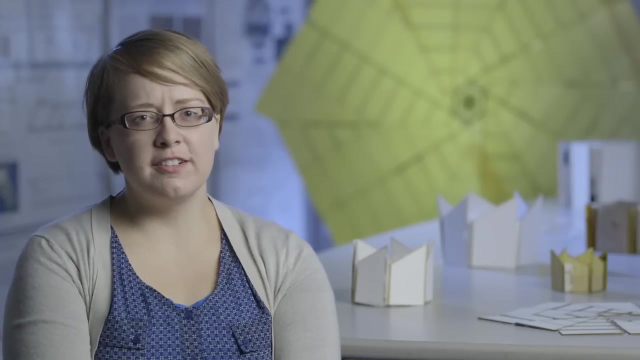 himself in this mathematics and origami kind of crossover field. And so this combination of taking this art, this ancient art, and combining it with engineering, we've been able to discover new things and new motions that wouldn't otherwise be possible. I think the biggest thing to learn from this kind of research is that you can find inspiration. 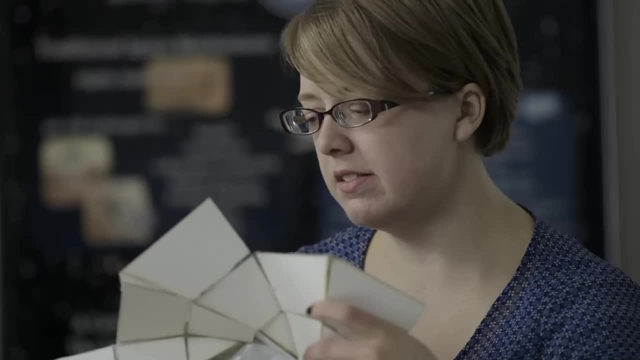 for designs from anything. If you're open to inspiration from any of these sources, then your creativity is not limited.